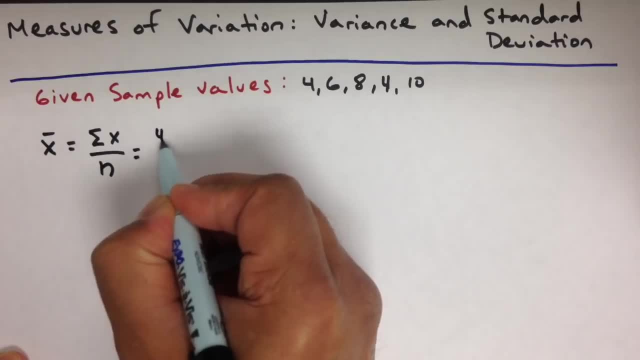 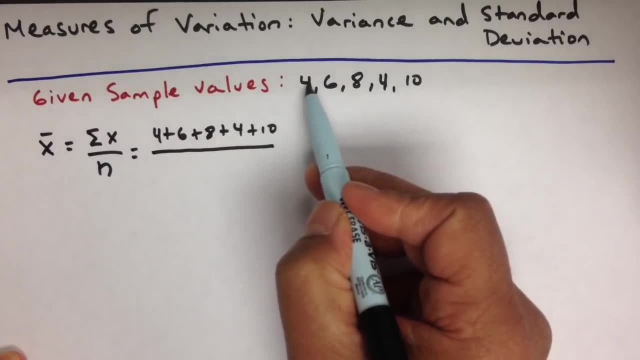 up So you can add up all of your samples. you can sum them all up, So four plus six plus eight plus four plus 10, divided by our sample size, While we collected one, two, three, four, five samples. So that's the size of our samples, That's the sample size. 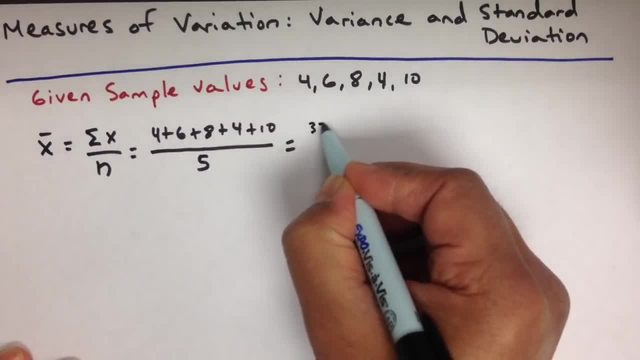 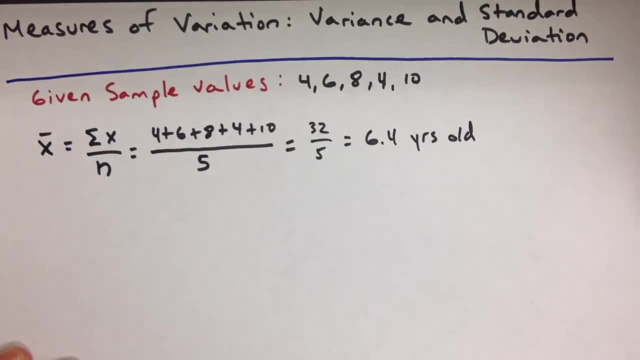 And you just use your calculator to do the math there. This will give you 32 divided by five, which gives us 6.4 years old. Or if you want to think about in terms of basketball, now let's, you can say that's 6.4 points per game. So let's check to see if we rounded this. 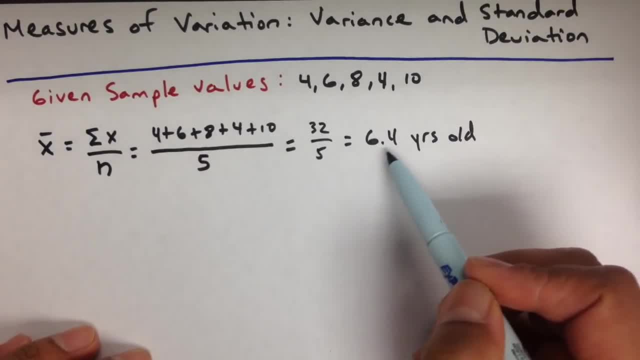 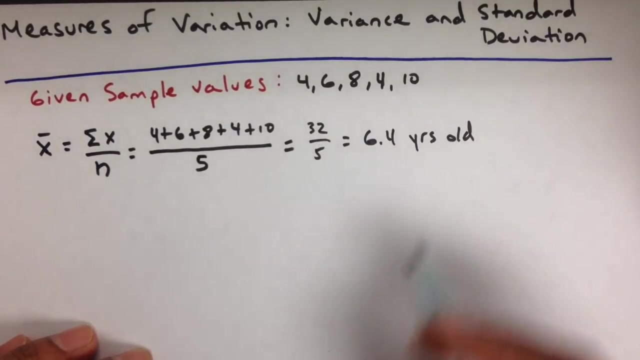 correctly. Well, we can only have one additional decimal place in our answer compared to our data. So, if you look, our data is all whole numbers. There's no like 4.1 or 6.25 or 8.356.. They're all whole numbers. So this is our one additional decimal place. If we had a 10.2. 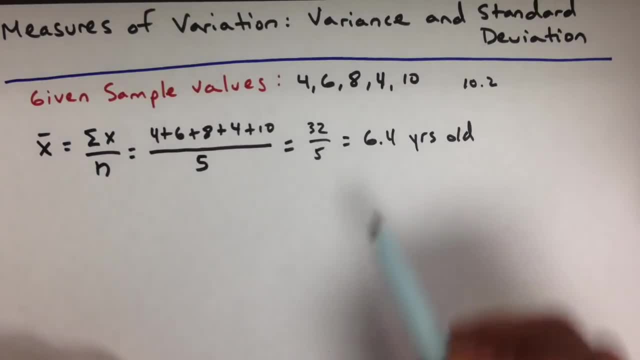 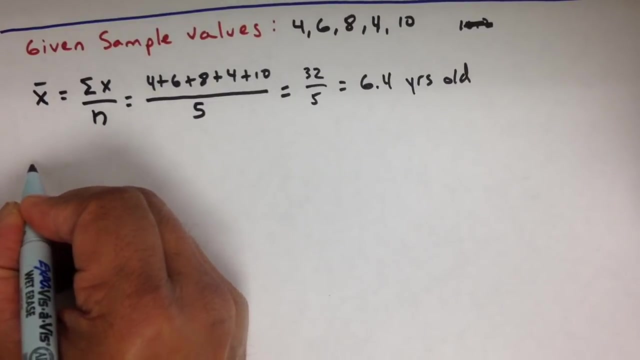 years old, then we could have an additional decimal place. here We can say 6.40, right, But for now, because we only have whole numbers, this is our allowed one additional decimal place. So sample standard deviation. we're going to call it sample standard deviation because it's based. 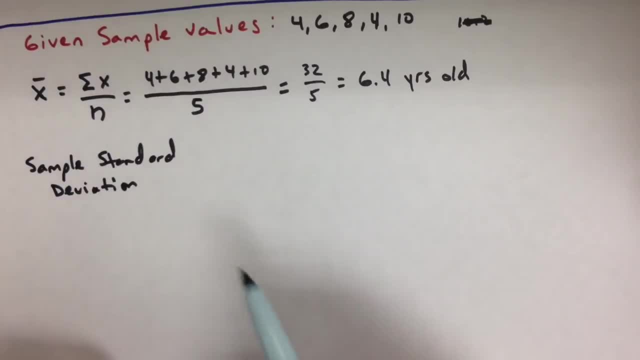 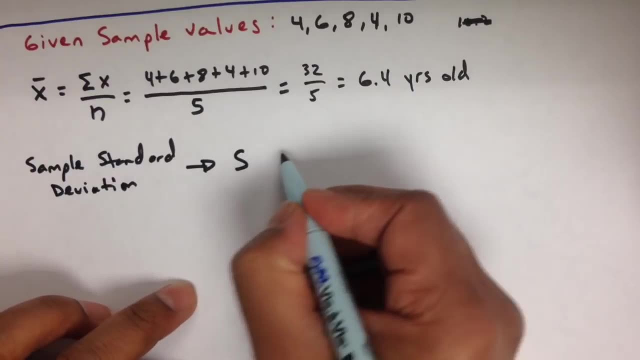 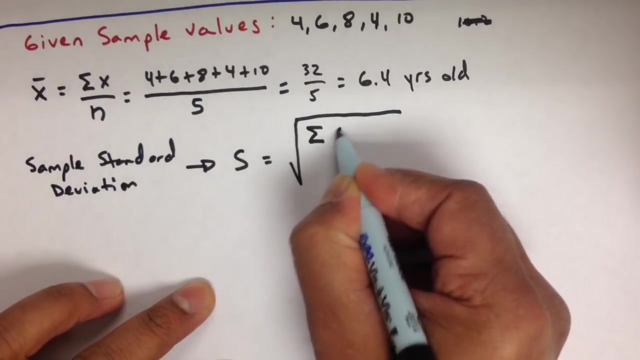 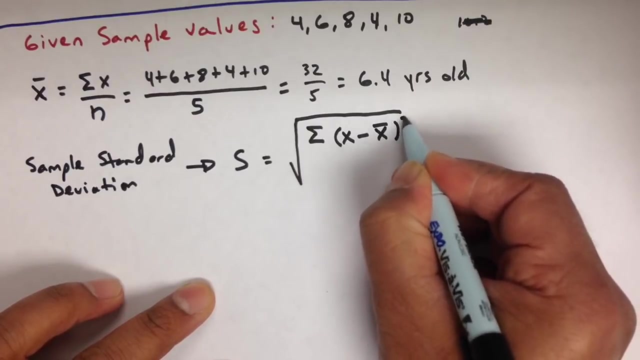 off a sample. The population standard deviation equation is going to be a little bit different, But this is our sample standard deviation equation And we use a simple S to represent that. So our sample standard deviation equals the square root Of the sum of our sample values minus the sample mean squared divided by n minus 1,. 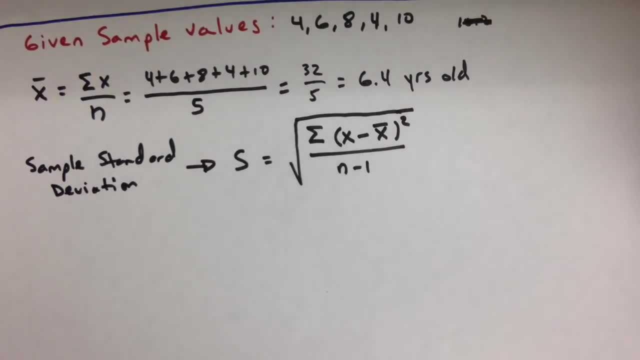 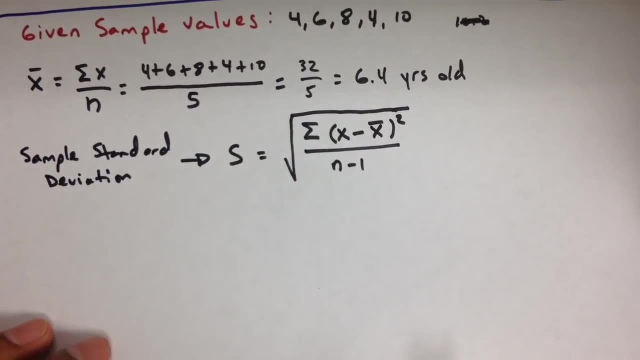 right: The sample size minus 1.. Now, don't get freaked out about this. It looks kind of crazy, but let's walk through a simple way of doing this by hand, in case you're asked to do that for a homework assignment. Obviously, this sort of thing would probably be easier on an Excel spreadsheet. 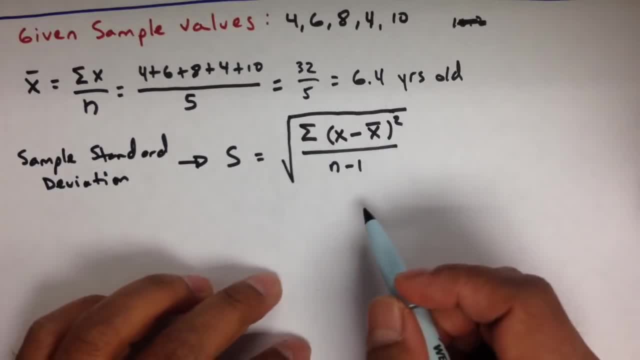 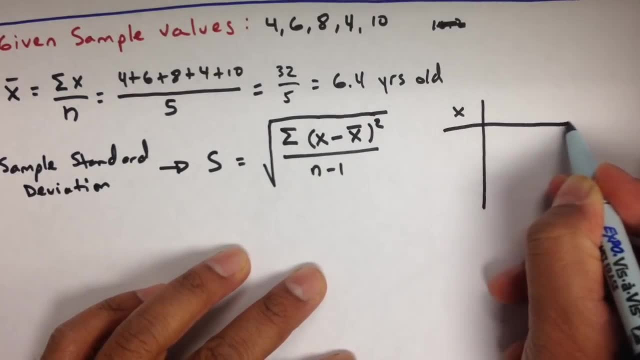 or some sort of computer. But if you're asked to do this by hand, what I recommend you do is you create a table In one column. we're going to list all our values that we collected from our sampling. So 4 years. 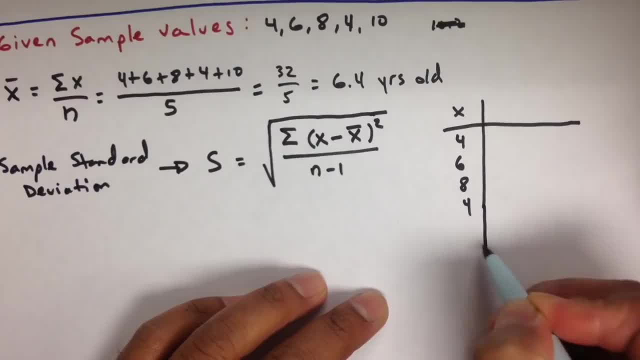 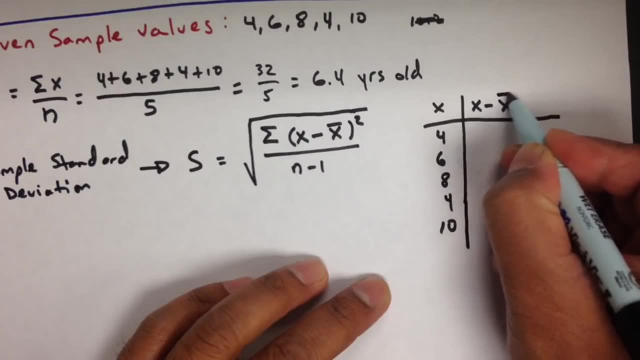 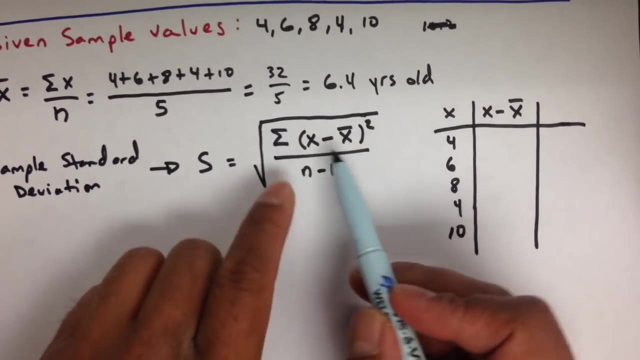 old, 6 years old, 8 years old, 4 years old, 10 years old. We're going to have a column for all of the x minus the means, minus the sample means. And why do we do that? Well, because we need a. 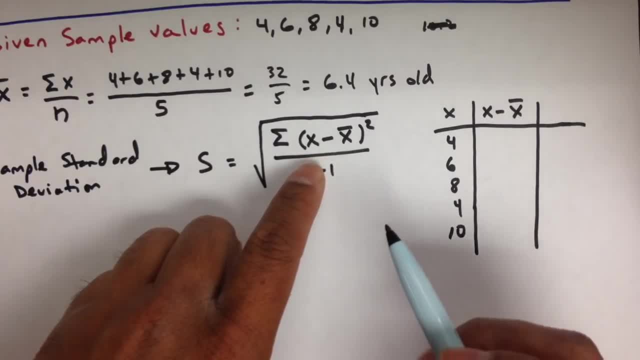 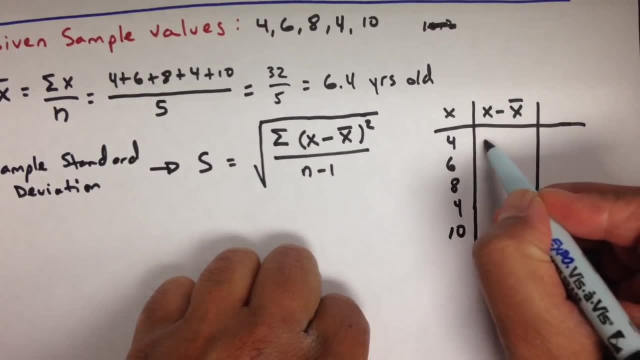 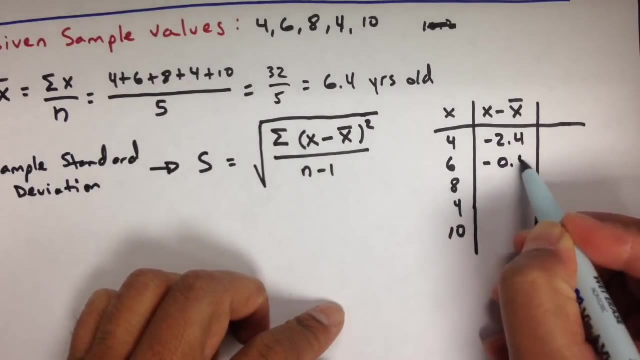 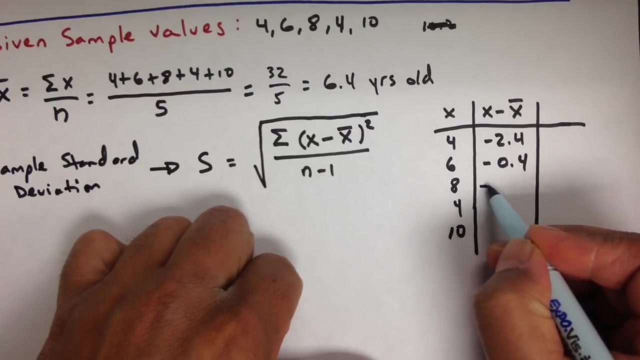 sum all of them up after we square them. So we need to get all those values. So 4 minus 6.4 is minus 2.4.. 6 minus 6.4 is minus 0.4.. 8 minus 6.4 is minus. I'm sorry that's positive is just 1.6.. 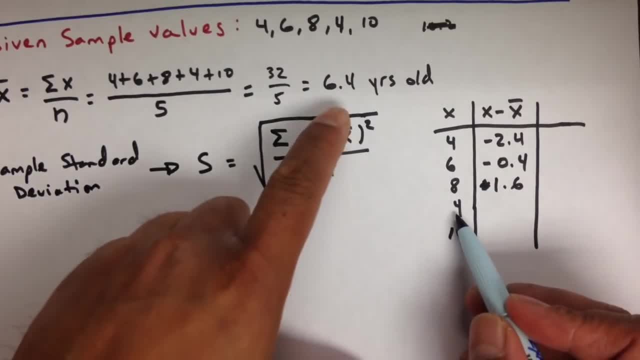 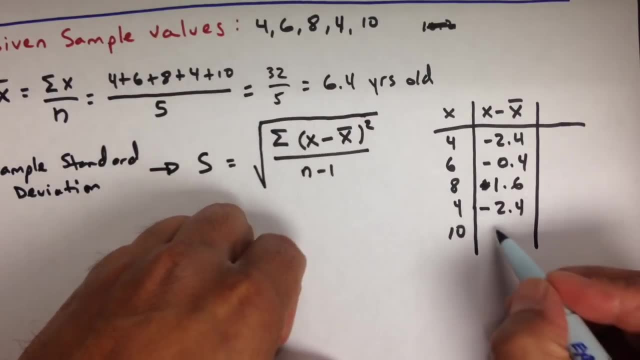 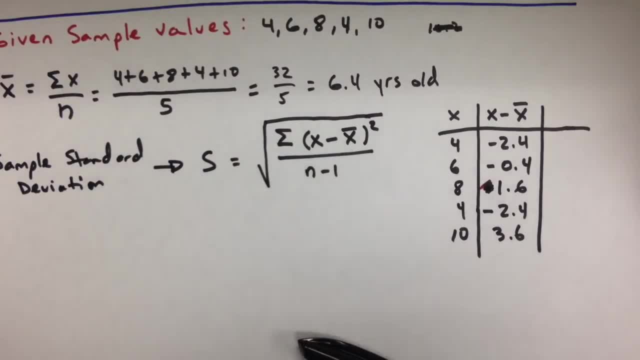 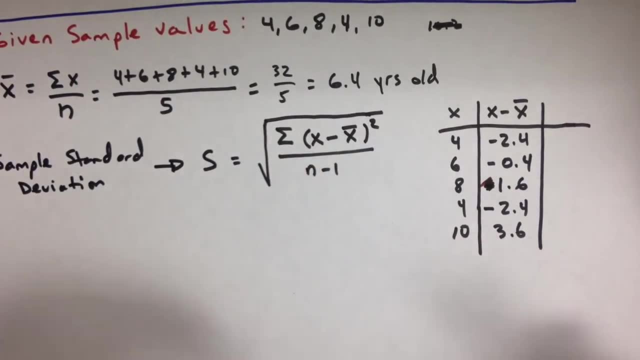 this guy. That's a mistake. OK, So what do we need to put here? then you think, Well, we eventually need to sum up all of those numbers after we square them. So let's go ahead and put a column of us squaring that number. 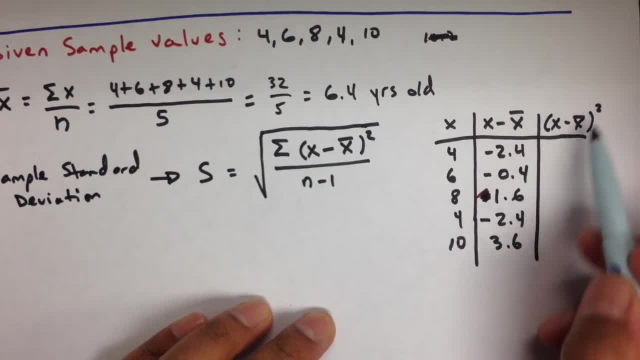 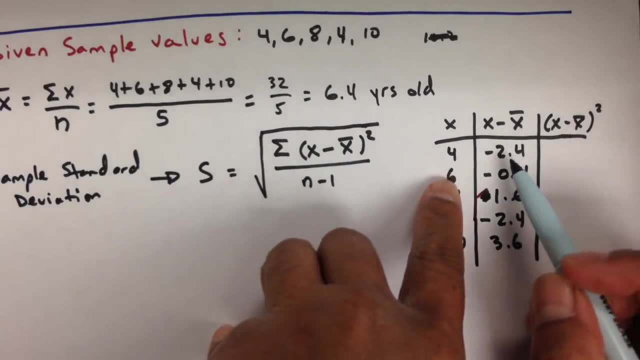 All right. So we're going to take this value and just square it x minus the mean. So these are all x minus the means. And now we're going to square all of those values. So in your calculator you would square 2.4.. You use your little square button Now you might. 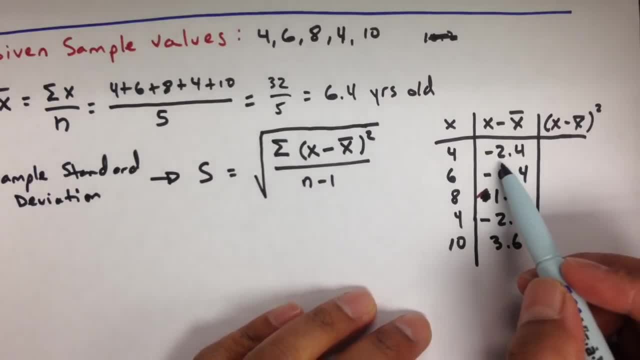 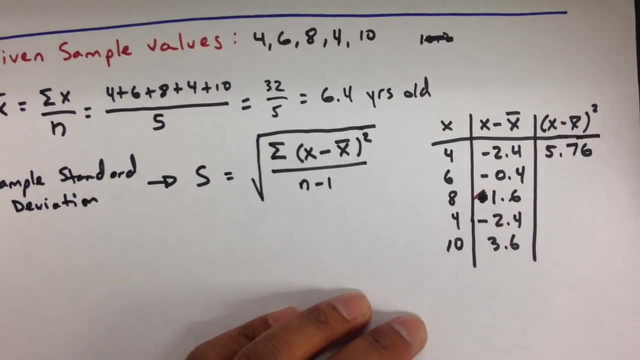 have an xy button in your calculator you can use too. So if you square minus 2.4, it's going to be a positive 5.76.. Remember, after you square something it's always going to be a positive number. 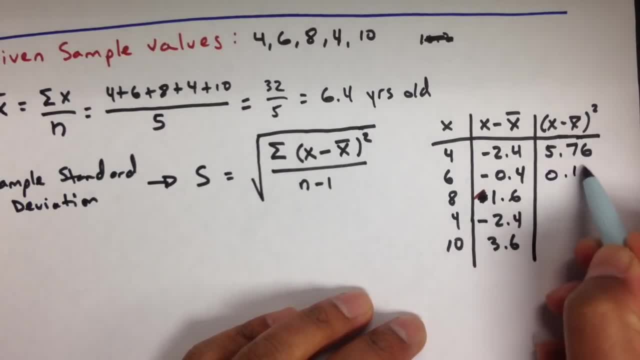 So negative 0.4.. 0.4 squared is 0.16.. 1.6.. The positive 1.6 squared is 2.56.. Negative, 2.4 squared is 5.76.. And then 3.6 squared is 12.96.. OK, So what do you think the next step is? Well? 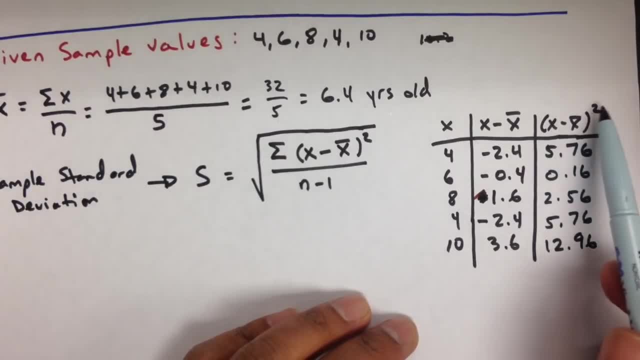 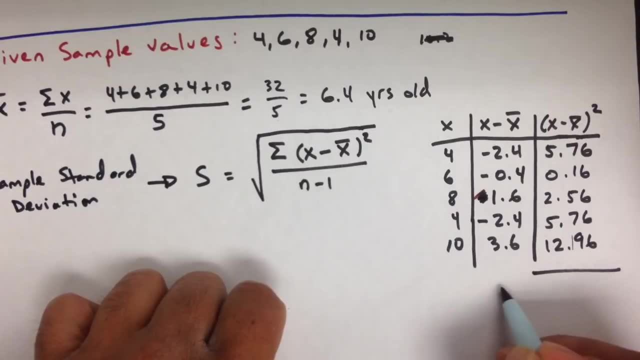 we've gotten all of it. We've calculated all of the x minus the means squared And we're told in the equation that we need to add them all up. So we need to sum this. So if we put the equation here, if we summed all of the x minus the mean squared, what? 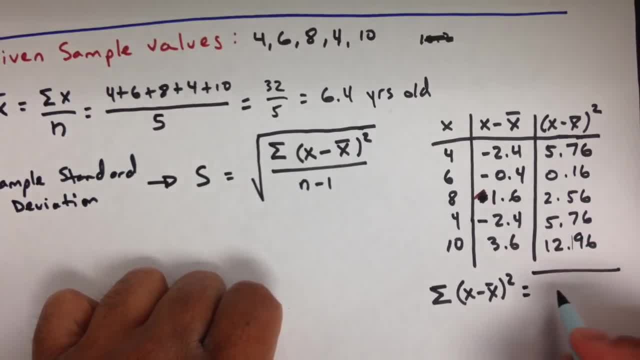 would it equal? Add these all up in your calculator and you'll see that it equals 27.2.. OK, And now we can put that number into that equation. So we have that. OK, We're going to add up the numbers. And now we're going to add up all of them. OK, And now we're going to add up the numbers. So we're going to give him the x, double the x and double the 2.2 squared. So we're going. 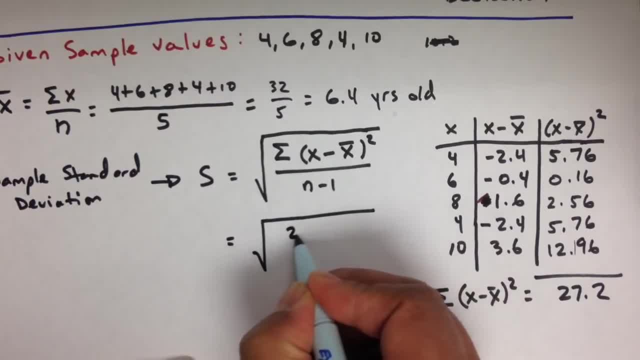 So we have the square root of 27.2 divided by our sample size, which is 5 minus 1, right? So obviously that's going to be 4.. So what you really have is the square root of 27.2 over 4.. 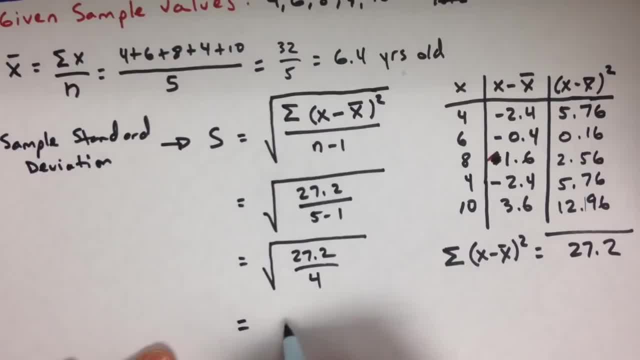 Okay, So that's about 2.6 and 0, 7.. You have a bunch of numbers And the units are years old for the years. But we have a round-off rule here, Remember, it's the same as the mean. 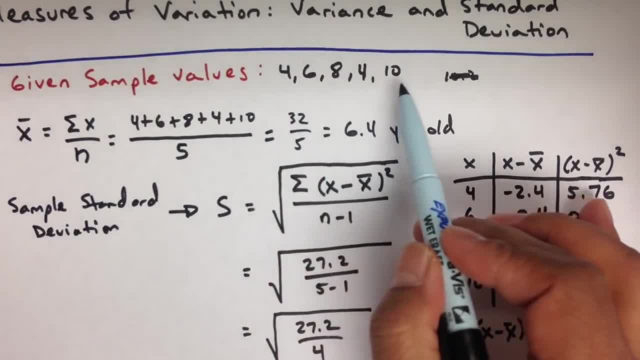 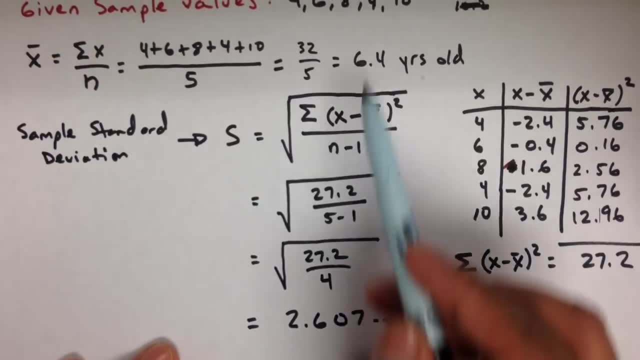 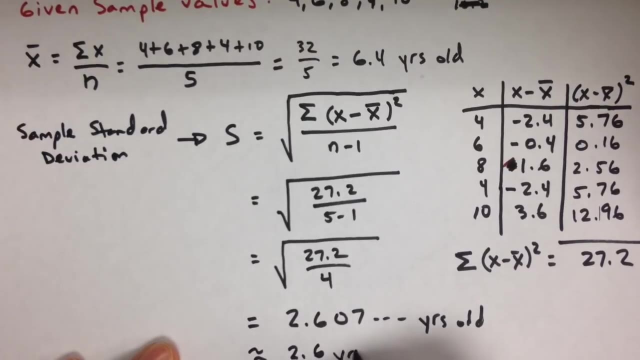 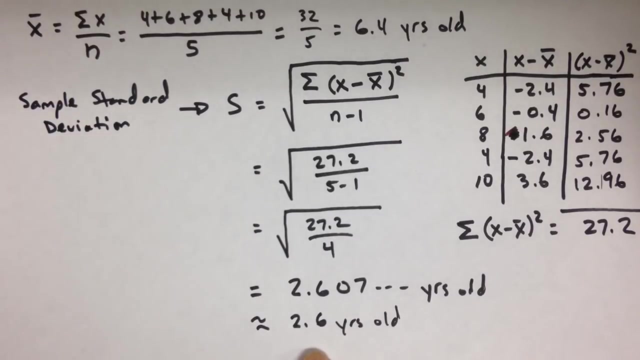 So if all our values in our data set are whole numbers and the rule is we can only have one additional decimal place as compared to our original data set, then this has to be rounded off to 2.6 years. Okay, So the average age- I'm sorry, the sample standard deviation of the kids at the party is 2.6 years. 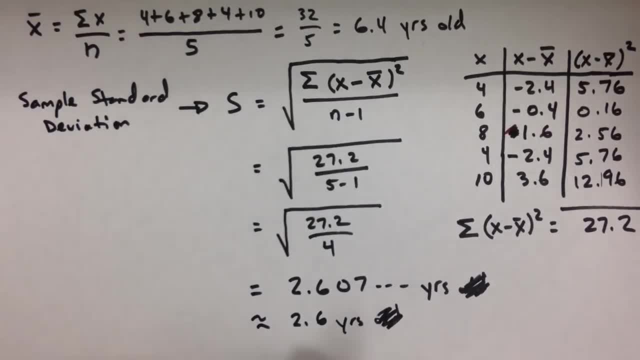 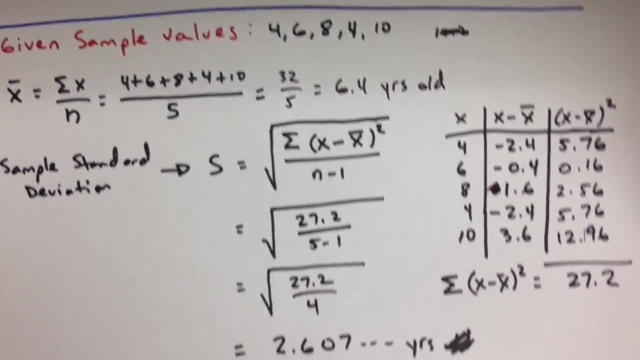 You don't have to say old. It doesn't really make any sense here. The average age is 6.4.. But in terms of how much this varies, the value we say is 2.6 years. That's the measurement. 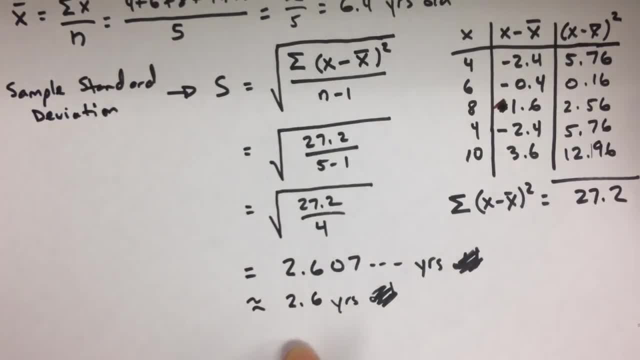 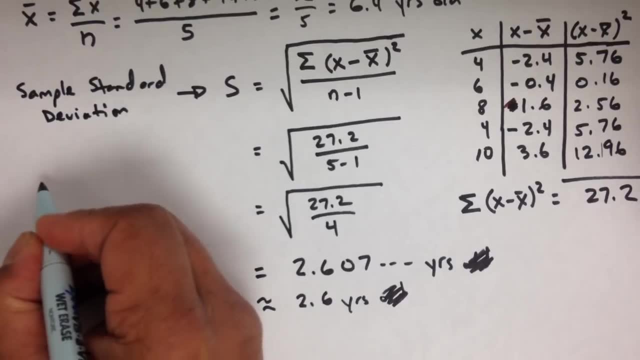 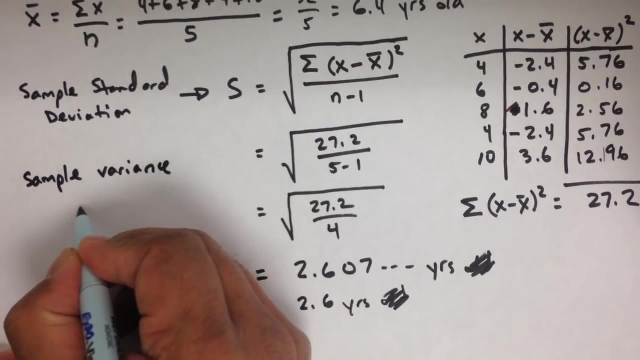 That's the variation standard through standard deviation. Now we also use variance to measure how much something varies. All right, Let's see, Let's put it over here: Sample variance. So the equation or the symbol for sample variance is just standard deviation squared. 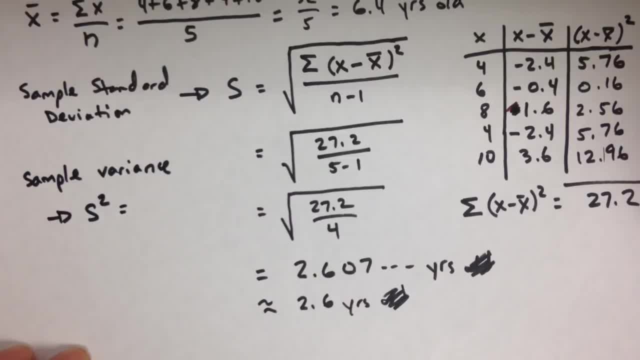 So we're going to take our standard deviation and just square it. So if you square the original value, it'll be 6.8 years and we're going to square it. Remember it's squared years because we squared this value. 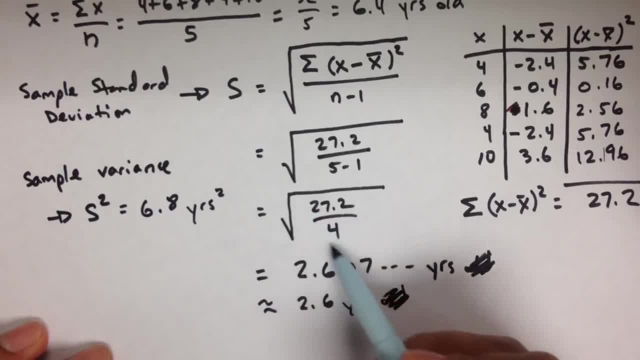 Now, if you think about it, what we really did is just we found this number right. We basically just found this value before we square rooted it. That's your sample variance, And the only reason you ever square root this to get standard deviation is because of the 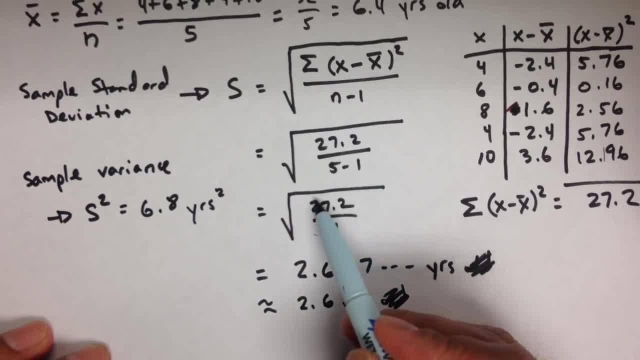 units 2.6 years, we understand, But the units in here remember this is a squared value, So the units are squared, Years squared. Well, have you ever heard of that used before? Have you ever heard anyone talk about years squared or points squared? 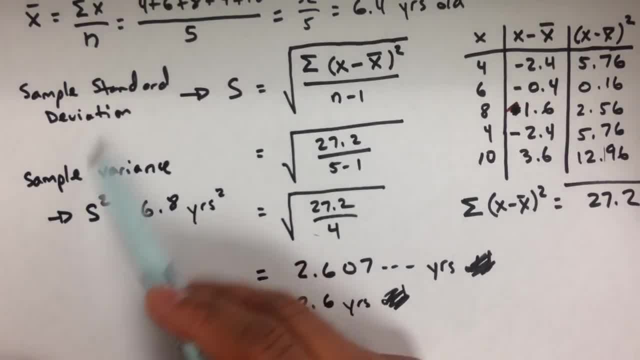 Not really So. this is why we use standard deviation often when we talk about how much something varies, because the units don't make any sense when we talk about variance- Years squared- That's kind of a weird thing to talk about. OK. 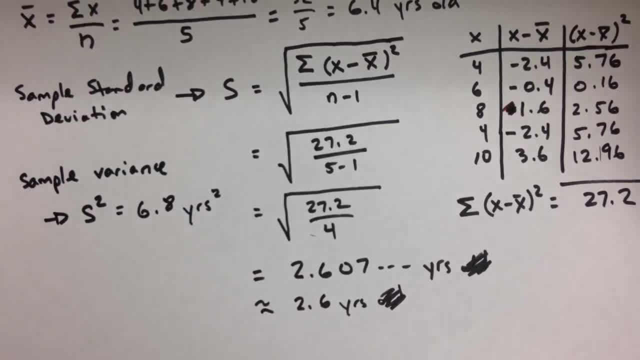 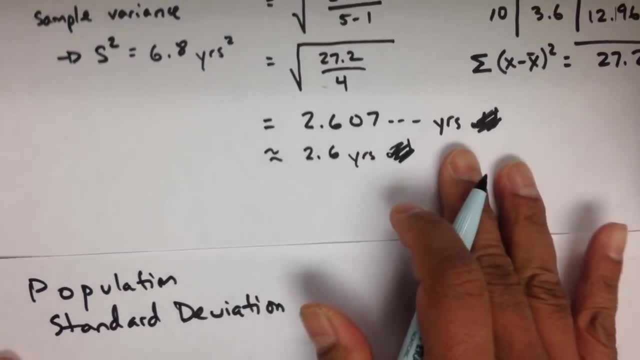 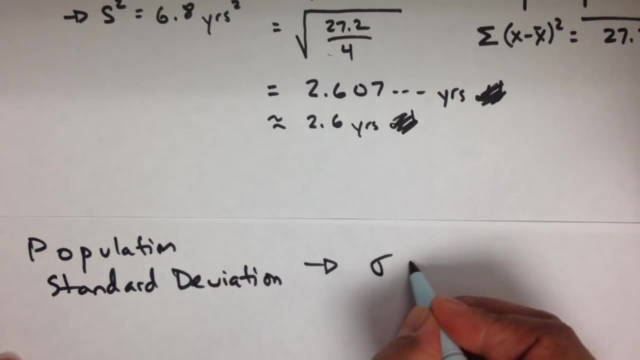 So how about population? What about population standard deviation and population variance? Well, it's really the same sort of equation. Let's take a look at it quickly. We have a different symbol now. The symbol is going to be sigma And the equation maybe on the surface might look different, but it's only because of notation. 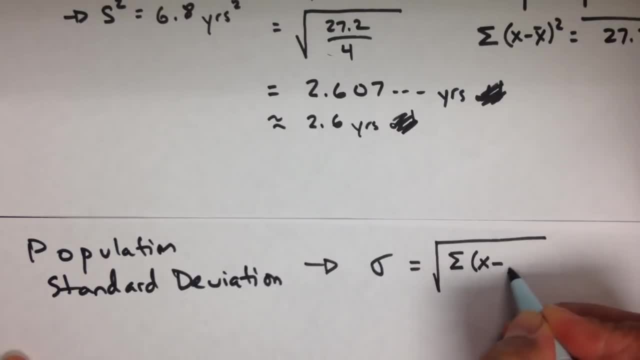 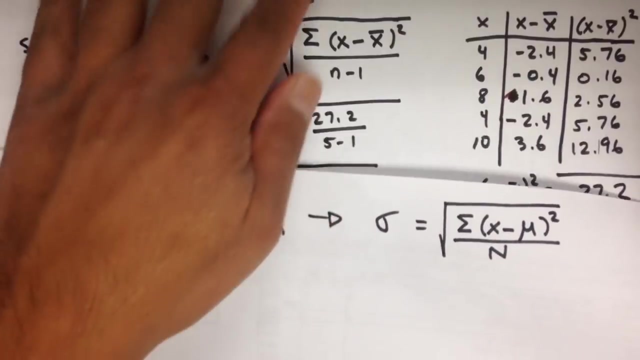 We're going to sum our sample values minus the population mean. We're going to sum our sample values minus the population mean squared divided by our population size. OK, So if we're going to relate it to what we just did a second ago, let's compare these. 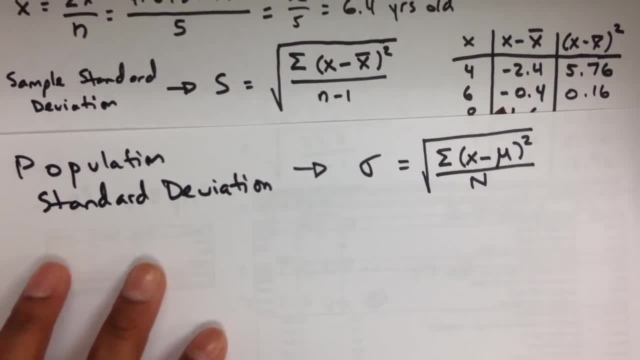 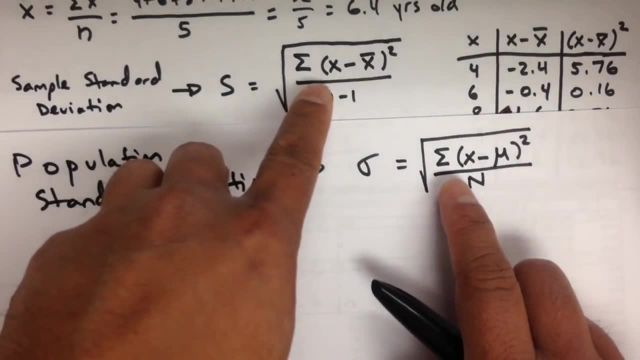 equations here. Here is our standard deviation for a sample, Here is our standard deviation for an entire population. You still have to sum up stuff, You still have to take into account your samples And you still minus the mean. But we just did that. 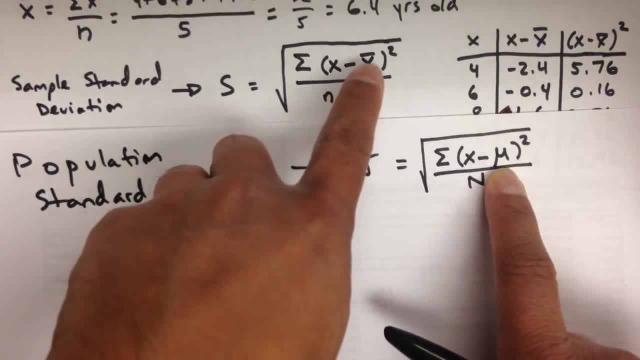 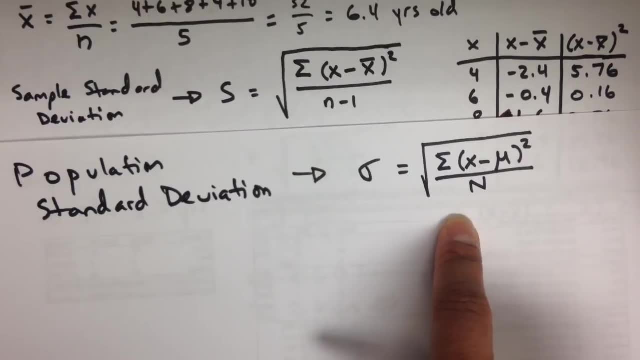 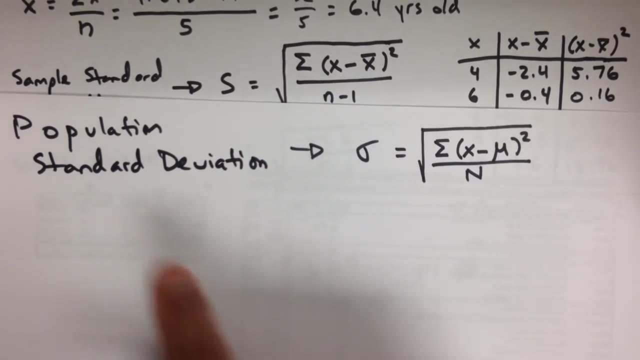 We just used different notation to note population mean versus sample mean And you still have to square stuff. And now we use the entire population here versus our n minus 1 for our sample there. So if you're trying to figure the population standard deviation for the same data set, 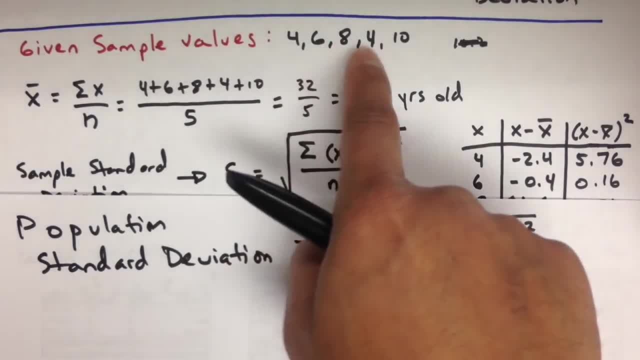 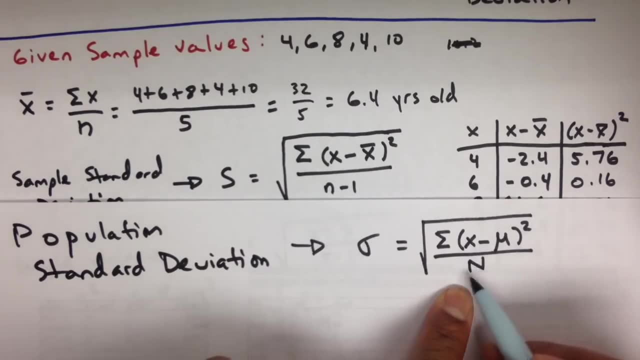 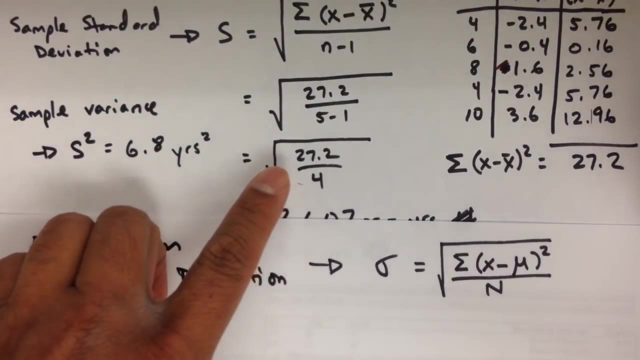 the same sort of scenario, assuming that we only have five kids at the party, right, That's an entire population, just five kids. Then you still use our same mean. But now this n equals 5, as opposed to having a 5 minus 1 in our denominator here. all right, 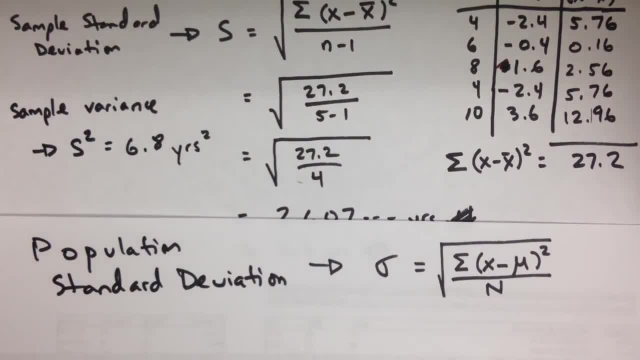 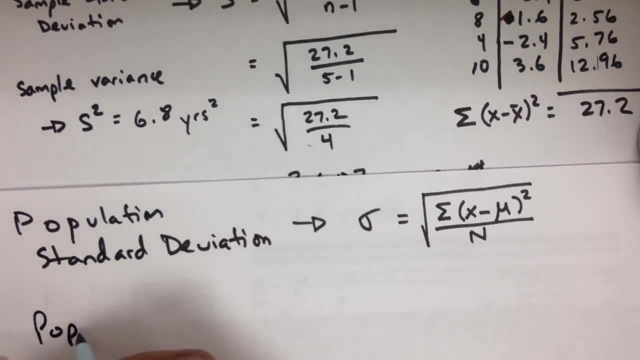 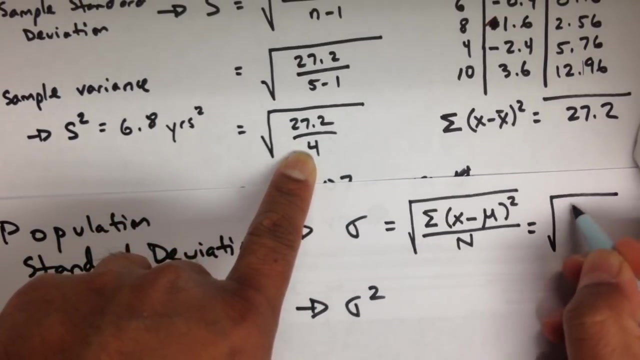 So it'll be the same sort of thing And then, just like with sample variance, our population variance is just our standard deviation squared. So, if you want to see this worked out, this value is still 27.2 using the same method we talked about earlier, right? 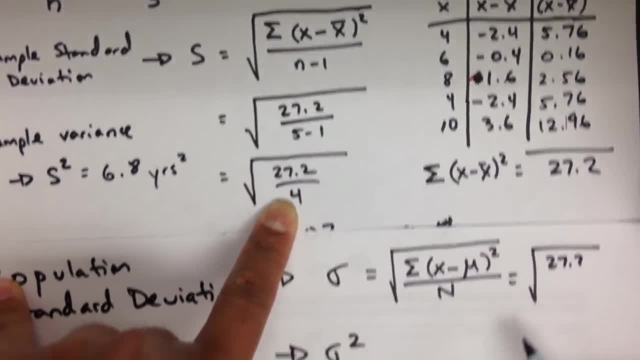 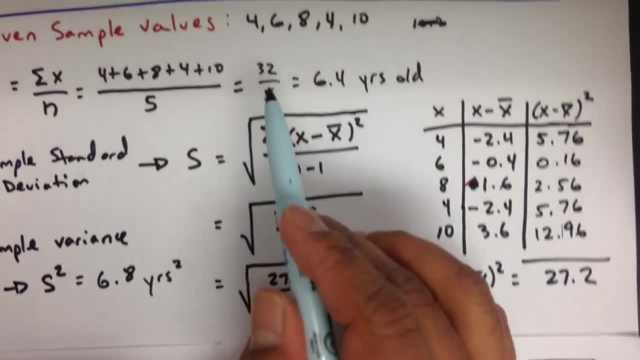 Using this method, using the table, But now, instead of dividing by 4, we're going to divide by 5, assuming that we only have five kids at the party, That means there's only five total. That's our population: only five in there. 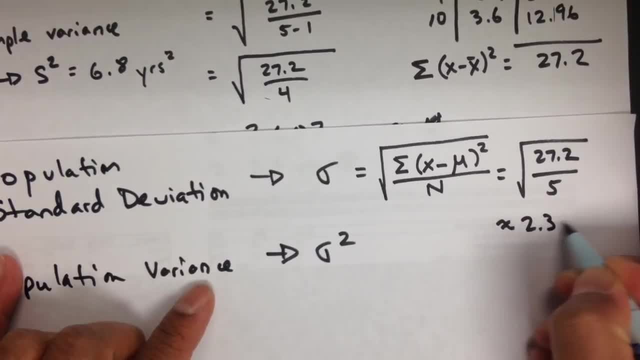 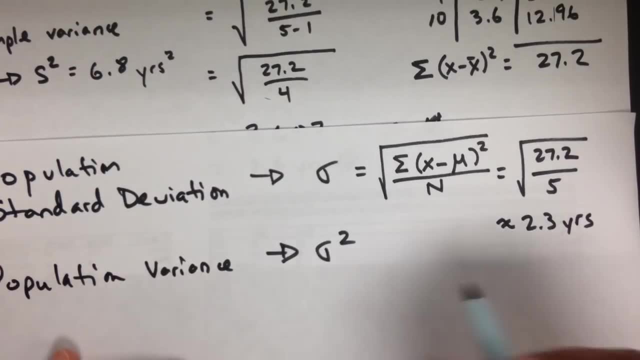 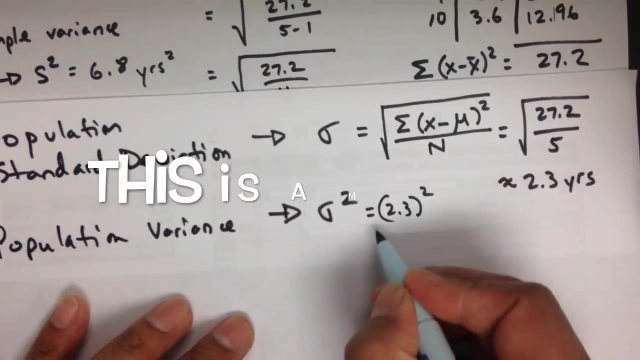 And this would give you 2.5.. All right, So that's 2.3 years and it's approximate, because I already rounded it off for you And then if you square that, you would calculate to square it. so 2.3 years squared equals.